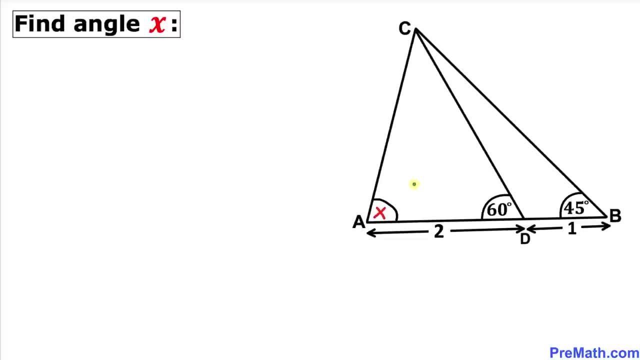 Welcome to PreMath. In this video we have got a triangle ABC, as you can see in this diagram, such that this line, segment AB, is divided into two segments in a ratio of 1 to 2, and, moreover, this angle B is 45 degrees and this angle D is 60 degrees. and now we are going to calculate. 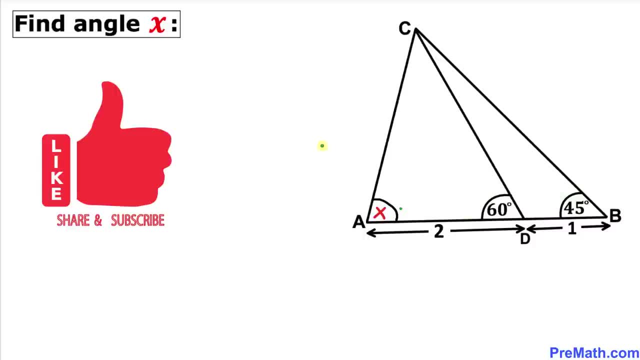 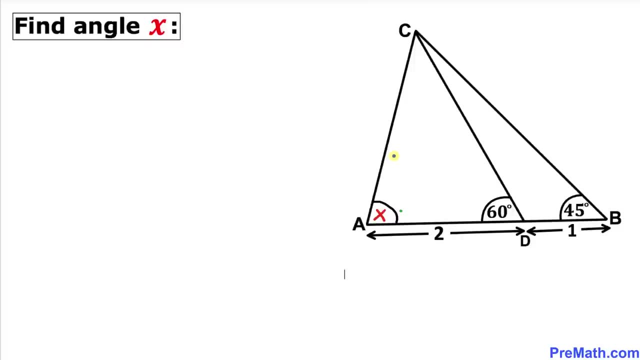 this angle X. Please don't forget to give a thumbs up and subscribe. So let's go ahead and get started with the solution, and here's our very first step. Let's look at this angle. that is 60 degrees, and we know this whole. 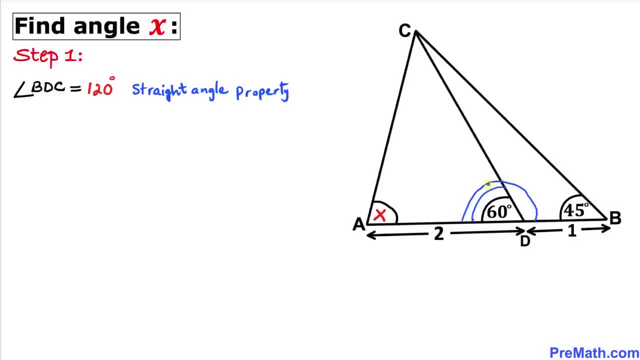 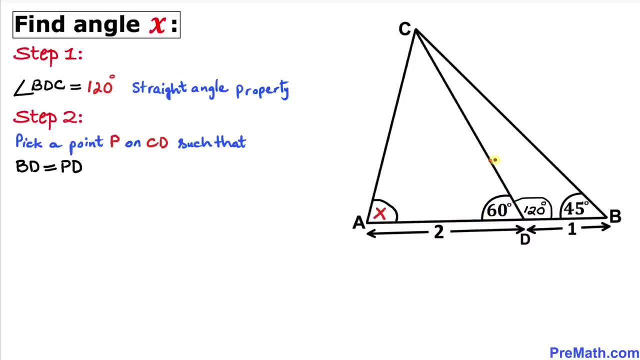 angle is 180 degrees. Therefore, this angle is going to be 180 degrees minus 60 degrees is going to make 120 degrees. No wonder I wrote down angle B. Ko is 120 degrees. And here is our next step. let's pick a point P on this line segment, CD, point P somewhere. 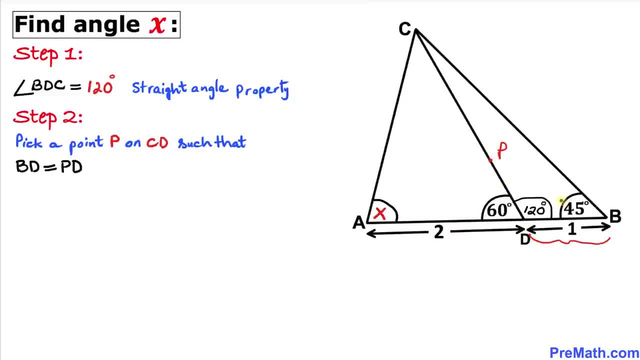 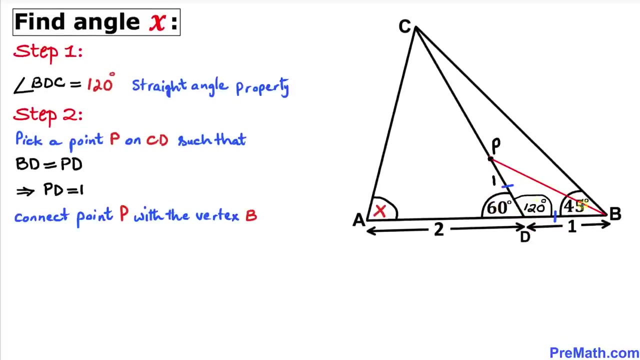 here, such that this line segment BD and this line segment PD are equal, and we know that this line segment BD is one unit. so therefore, this line segment PD is going to be one unit as well. and here's our next step: we connected these points P and this vertex B, as you can see over here, and 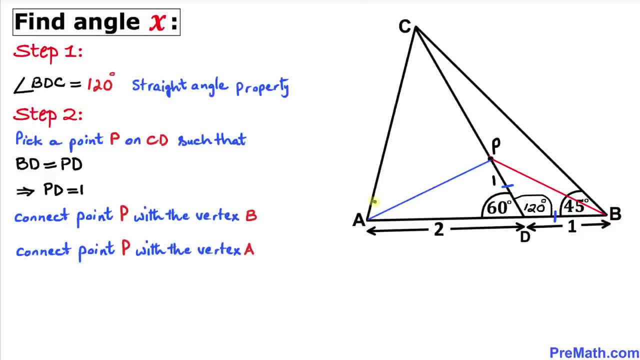 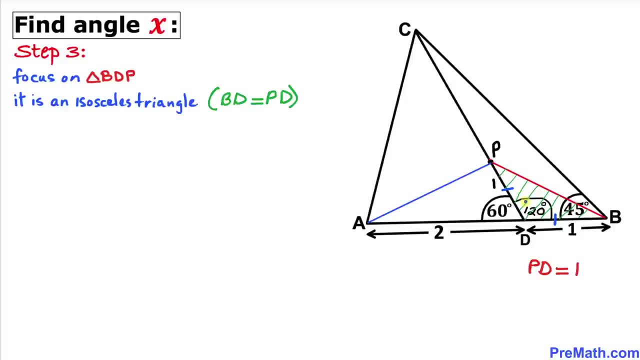 we also connected this point P with this vertex A as well, as you can see. and now here's our next step. let's focus on this triangle, BDP, and we know that this is an isosceles triangle, since this side length BD equal to this side length PD. so therefore this angle has got to be equal to this angle. so 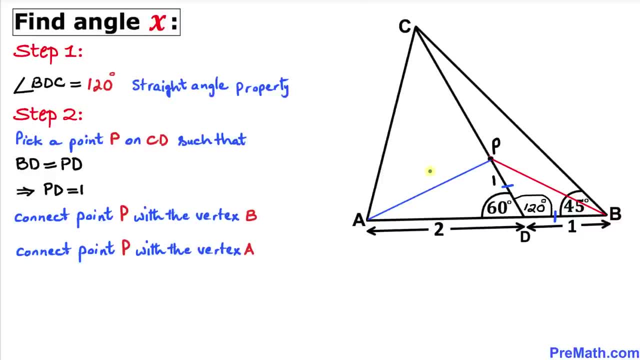 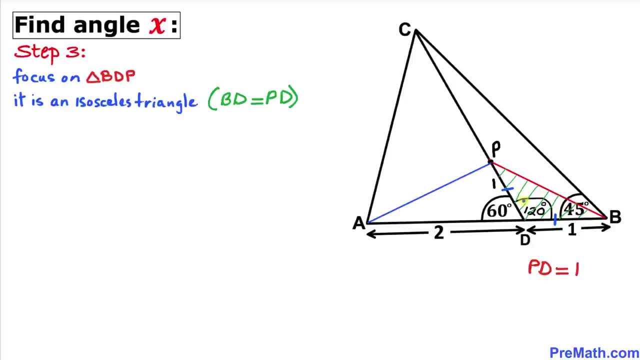 and we also connected this point P with this vertex A as well, as you can see. and now here's our next step. let's focus on this triangle BDP, and we know that this is an isosceles triangle, since this side length BD equal to this side length PD. so therefore this angle has got to be. 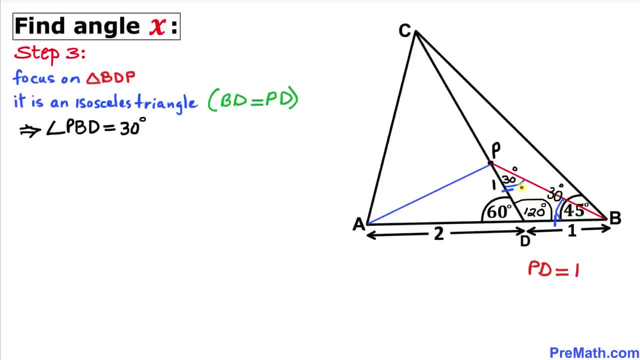 equal to this angle. so, therefore, this angle has got to be equal to this angle. so, therefore, this angle has got to be equal to this angle. so, therefore, these two angles, this angle and this angle, have got to be 30 degrees each, since the sum of these three angles, 120 degrees, this one, 30 degrees and 30 degrees, is going to. 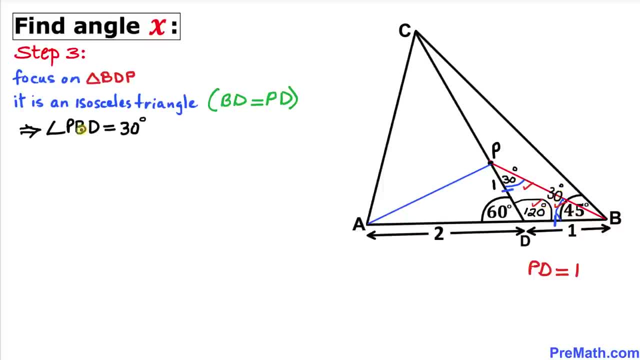 make 180 degrees. no wonder I wrote down: angle PBD is 30 degrees and, moreover, this angle PBC is going to be 40, is going to be 40 minus 30 equals to 15 degrees. and in this next step, let's focus on this triangle. 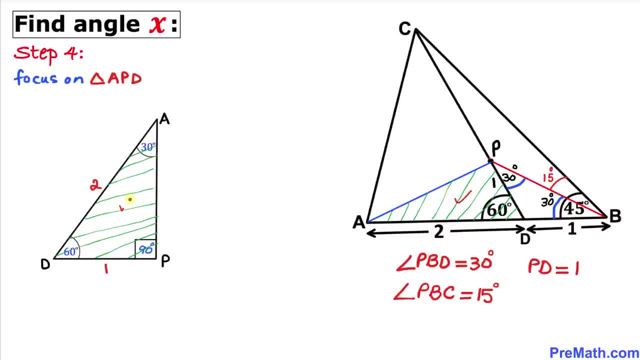 APD and I have here copied down this triangle over here. we know that this side length is one unit and this side length two unit. then we can see that this is a special 30, 60, 90 triangle. so therefore this angle P is equal to this side length and this side length is equal to this side length. 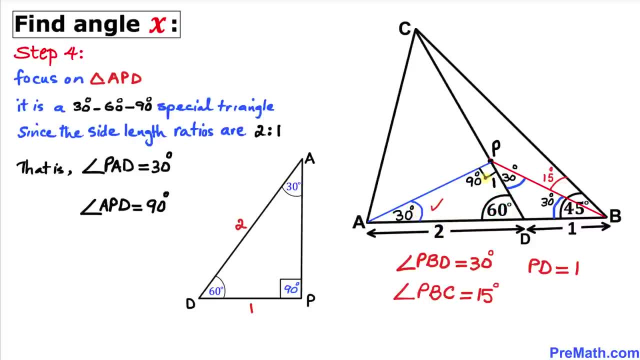 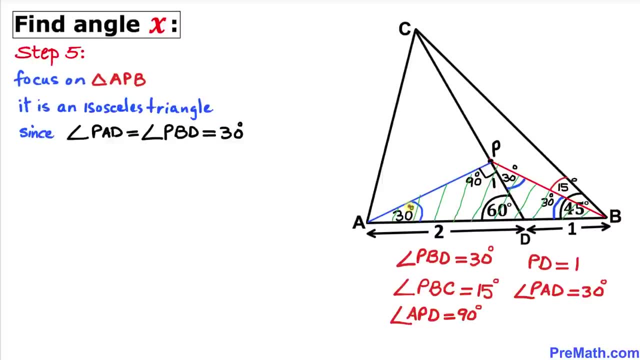 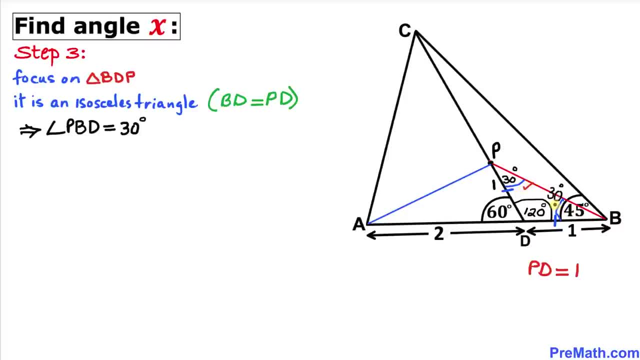 therefore, these two angles, this angle and this angle, have got to be 30 degrees each, since the sum of these three angles- 120 degrees, this one, 30 degrees and 30 degrees- is going to make 180 degrees. no wonder i wrote down angle pbd is 30 degrees and, moreover, this angle, pbc is going to be: 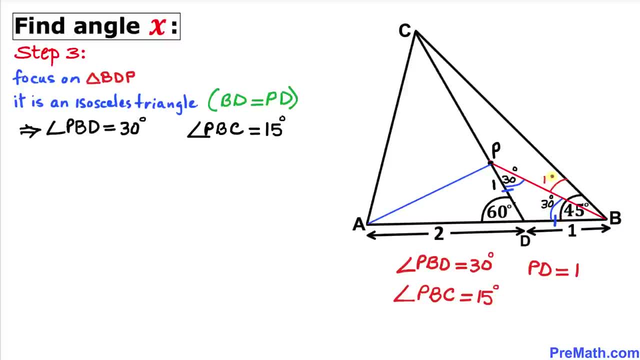 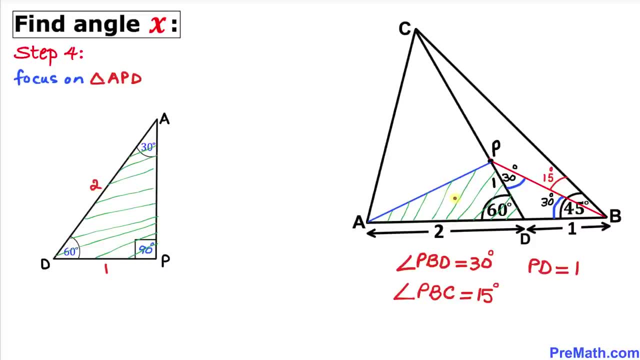 45 minus 30 equals to 15 degrees. and in this next step let's focus on this triangle apd- and i have here copied down this triangle over here- we know that this side length is one unit and this side length two unit. then we can see that this is a special 30, 60, 90 triangle. so therefore, this angle, 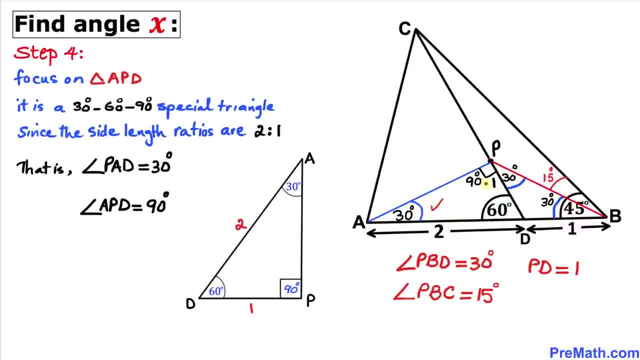 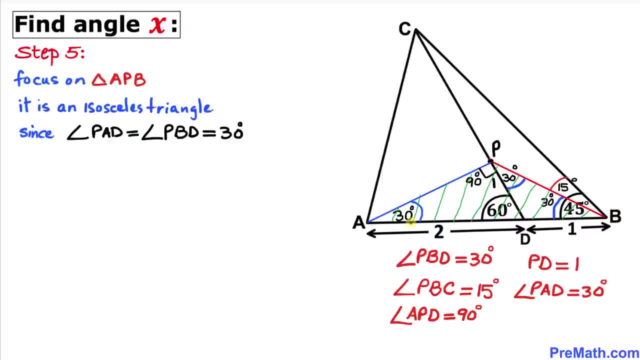 pad is going to be 30 degrees and this angle, apd, is going to be 90 degrees. and now let's focus on this triangle, apb. and we know that this is an isosceles triangle, since this angle is 30 degrees and this angle is 30 degrees as well. so therefore, we conclude that these side lengths ap. 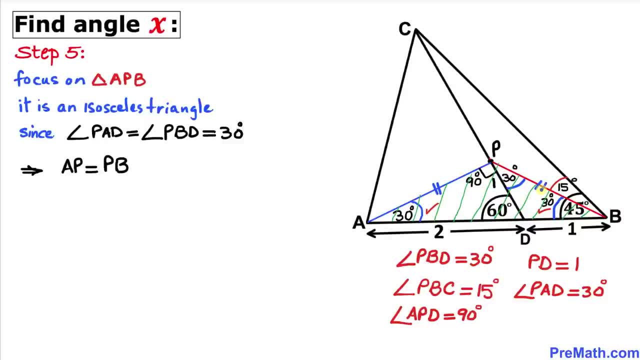 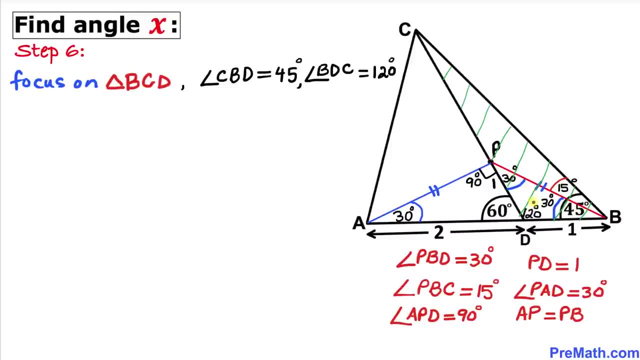 this side, length, pb are equal in length. and now, in this next step, let's focus on this triangle bcd. we know that this angle is 45 degrees and this angle is 120 degrees, and we also know that the sum of the angles in any triangle is 180 degrees. so, therefore, our this angle. 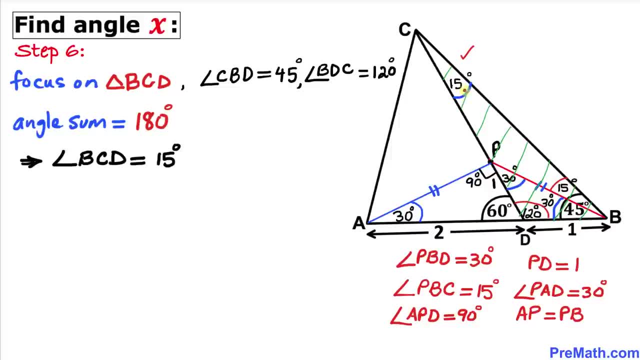 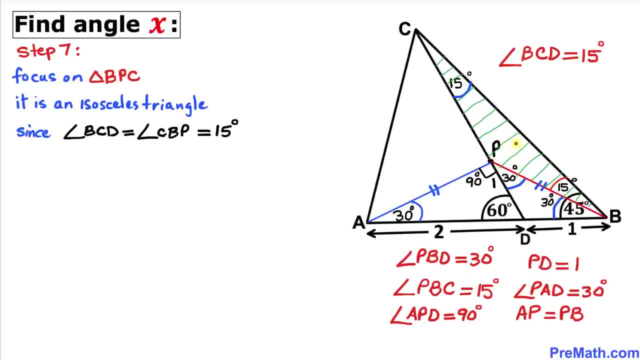 bcd is going to be 15 degrees. and now let's focus on this triangle bpc, and we know that this is an isosceles triangle, since this angle bcd and this angle cbp, both of them are 15 degrees each. therefore, we conclude that these side length bp and this